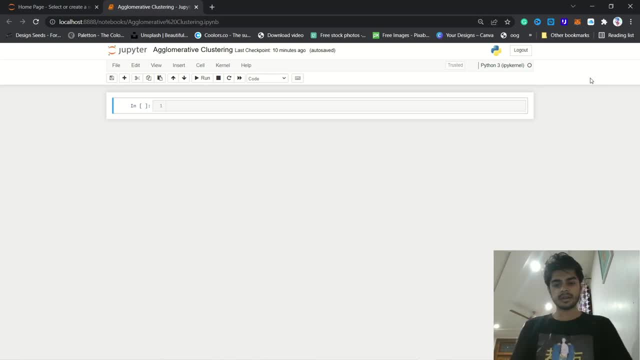 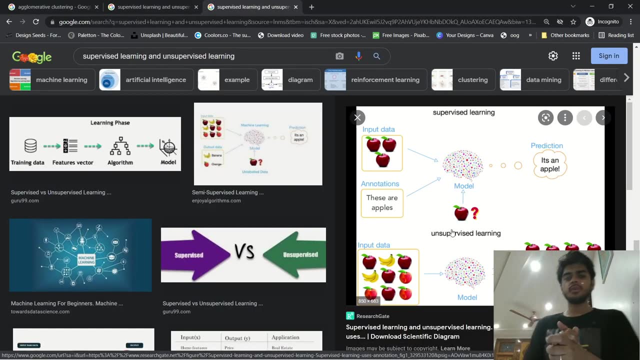 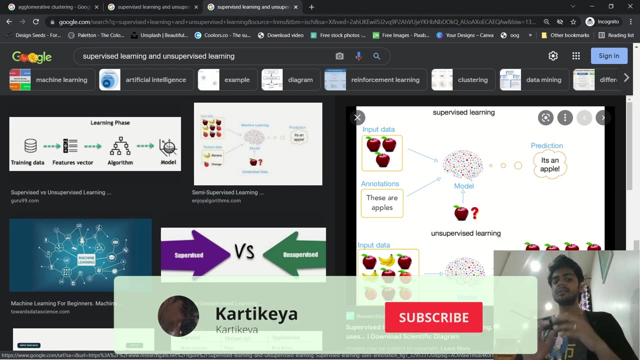 why we use clustering. So I have actually opened a Chrome where I have this diagram. So, as you can see in this picture, you can see the difference between supervised learning and unsupervised learning. The basic difference and the key difference between supervised learning and unsupervised learning is: 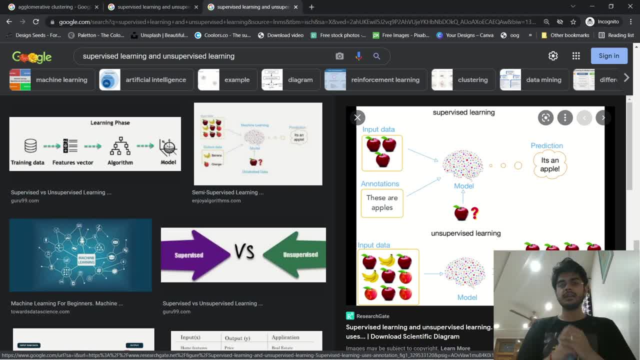 that supervised learning have a label, has a label with the data. Let's say we have an input data- Apple, there will be an annotation that these are apples. then we feed these label and input data into machine learning model and it predicts whether it is Apple or not. On contrary to that in unsupervised learning, 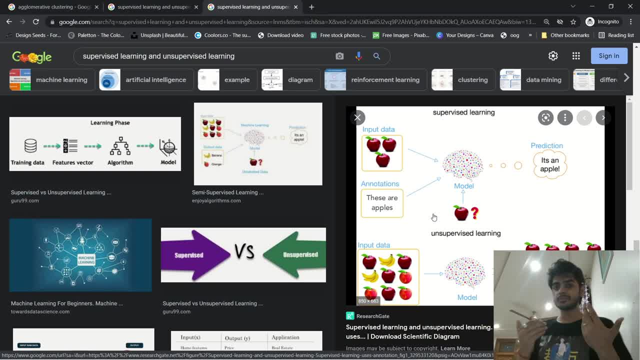 there is no label. that is a key difference between supervised learning and unsupervised learning. So Ensupervised learning comes with the label and unsupervised learning is learning doesn't have any label. So, as you can see, in unsupervised learning they 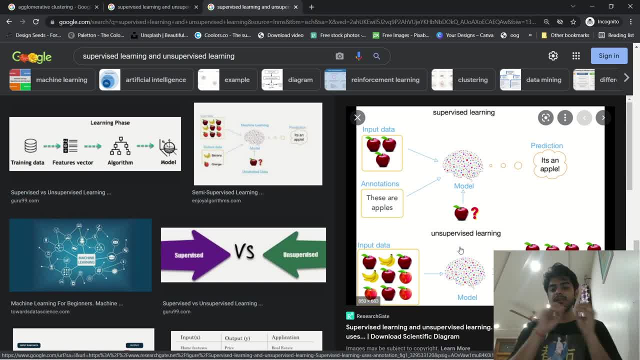 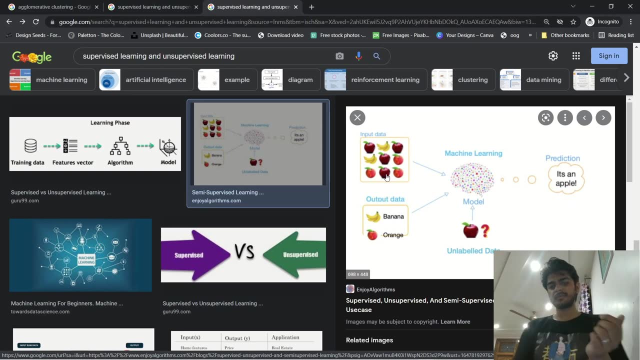 have banana, we have Apple, we have oranges. We feed that into machine learning model. machine learning model predicts whether it is a apple or an orange and banana or banana. how So? if I go back, there is this picture which explained this in a little more detail: In unsupervised learning. 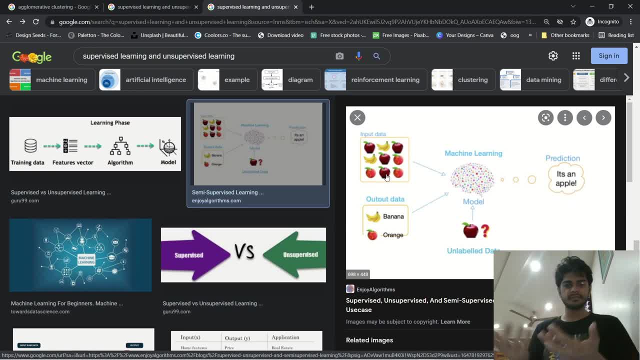 learning. we get an input data of apple, banana and oranges. this is an example which i'm taking and we have an output data which tells us that, okay, this is a banana, this is an orange. but there is one more data point in our input data which is an apple and it is like not labeled. we have 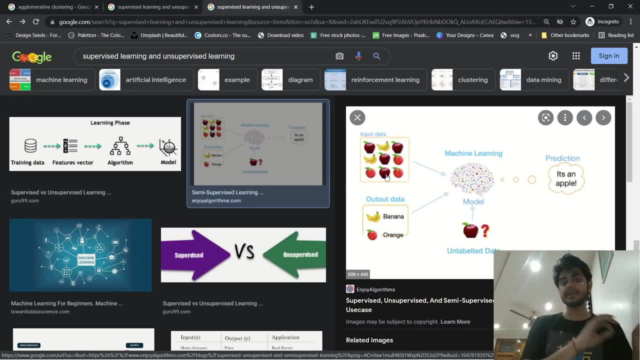 nothing which explains that this is an apple. so what machine learning do, unsupervised learning does, is that it takes banana and it takes- uh, it takes- whole input data and it like keeps on dividing it to single point, whether, where he can, where it can check it is apple, oranges or 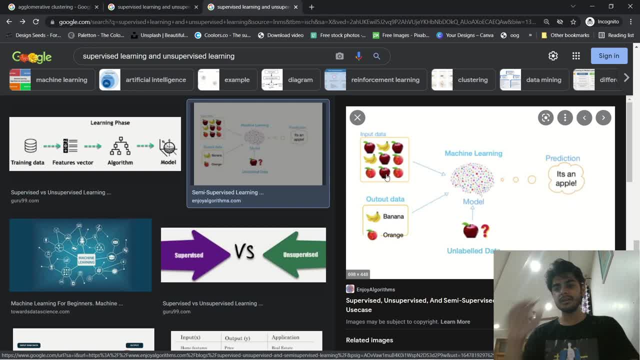 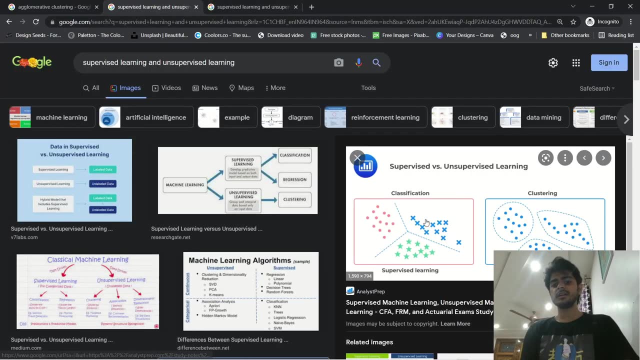 banana. so by this property, unsupervised learning get to know whether it is an apple, banana or an orange. to explain it. it move further. so here it is, in just a second. in supervised learning we use the algorithm classification, we classify the, our data with uh labels. on contrary to that, in unsupervised learning we uh use a clustering method. what is? 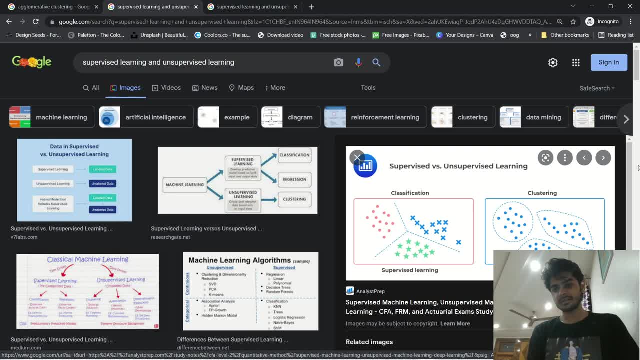 clustering. as you can see that here is a data point. let's consider this as whole as our input data. so we made a cluster of this data. we made a cluster of this data. we made a cluster of this data and after, like, when we feed this into our machine learning algorithm, uh, or it will take all this data and 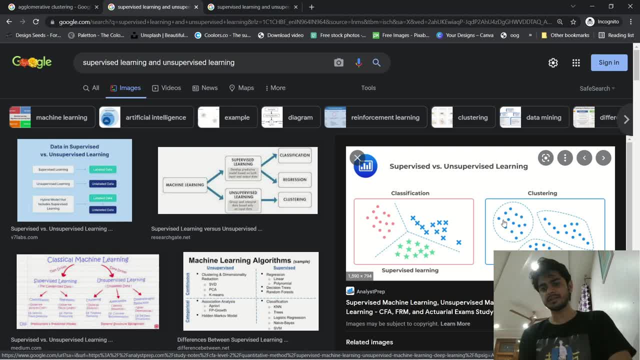 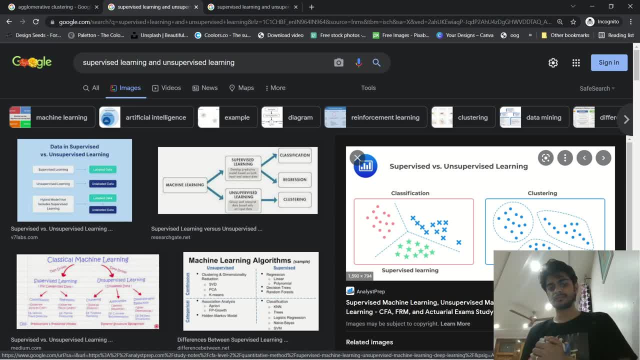 this is an apple, this is a banana and this is an orange. so, um, if we are taking our example, so, uh, how many types of clusterings are there? so clustering is generally divided into two parts, which is, uh, our agglomerative clustering, or which is our, um, hierarchical clustering and agglomerative clustering. and we 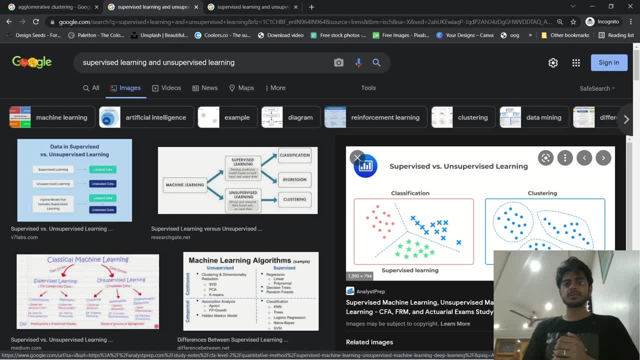 have a partial of partitional clustering. so what is agglomerative and what is partitional clustering? so, uh in, uh, our hierarchical, uh, hierarchical or agglomerative clustering? uh, we have overlapping of data, like we have a data which overlap with each other and we divided that data hierarchically, while in our partitional clustering, 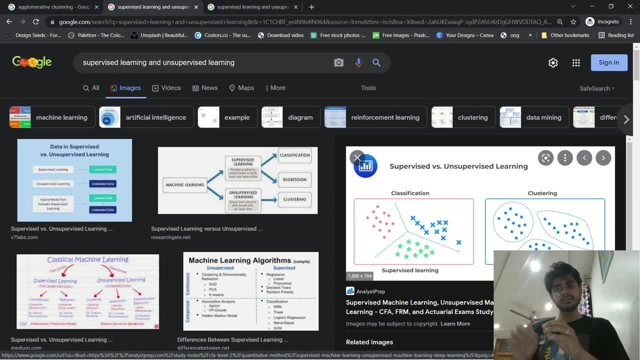 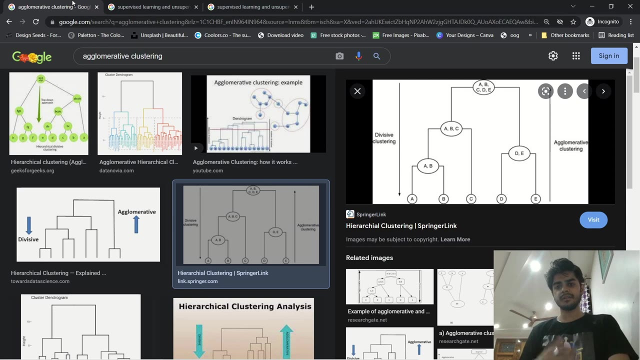 there is no overlapping of our data. so in partitional clustering we have algorithms like k-means, fuzzy mean, and in our this hierarchical, hierarchical clustering, we have have our agglomerative clustering and divisive clustering. So let's check what is agglomerative clustering and how divisive clustering works. So in our hierarchical clustering you can: 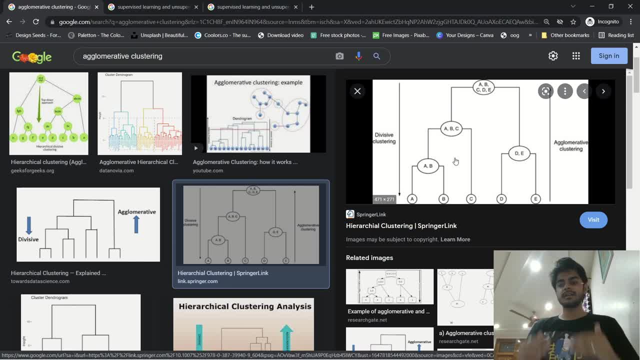 see that this is a hierarchy of things. Hierarchy is, let's say, if I have to take an example, let's say you have your family tree. Your family tree is like your grandparents, then your parents, then you and your siblings and everything, So that tree divides into a hierarchy. 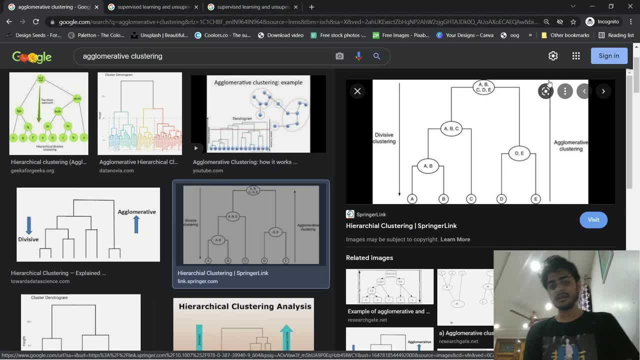 then it divides into a hierarchy and that divides into a hierarchy. This figure is known as dendogram. Like this thing is known as dendogram. So, as you can see that divisive clustering and agglomerative clustering are just reverse of each other, This whole thing is known as hierarchical clustering because it is representing and. 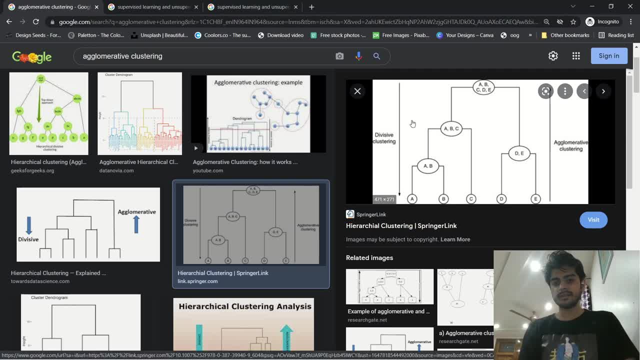 it is in the form of hierarchy, But in divisive clustering. we have our whole data set. then we divide that data set into two parts or n parts. then we divide this part into n parts, this part into n parts. then we divide this part into n parts and this part into n parts. 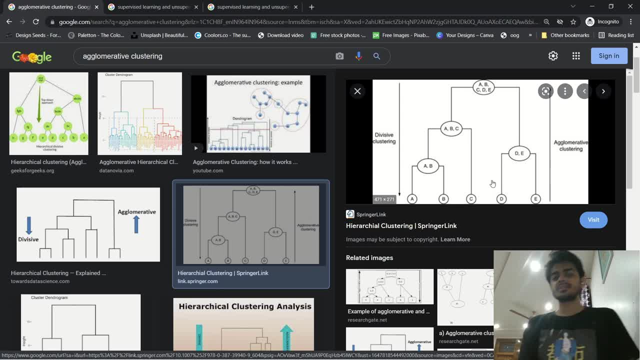 and can be any number based on the size of your data set. So In divisive clustering we divide data like from bigger to smaller till singularity. In agglomerative clustering we have single data points which we merge with each other to get a bigger picture. Let's say in agglomerative clustering we will like, take a, b and we will. 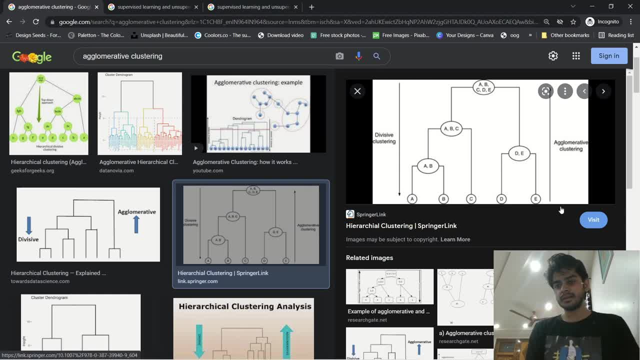 make it one. then we will take a, b, c and it will be one, d, e with one, and then we will add these two to get a bigger picture. So I hope now you have a basic understanding of what is supervised learning and what is unsupervised learning. 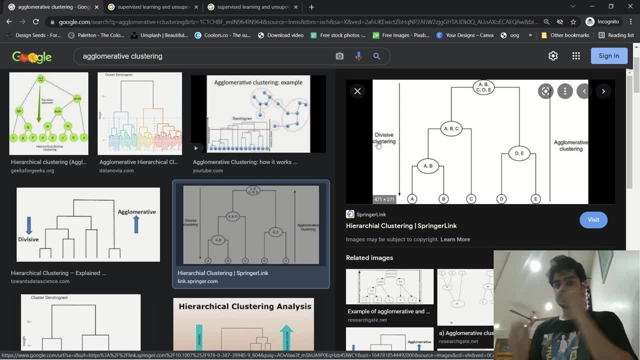 what is hierarchical clustering? what is partition clustering? We will code partition clustering also, but in this video we will code agglomerative clustering, which is form of hierarchical clustering. In hierarchical clustering we have agglomerative clustering and we have divisive clustering. and then in our partition clustering we have 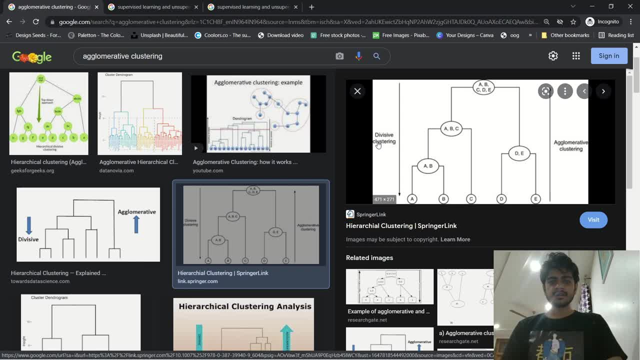 fuzzy k-mean, Fuzzy c main. so this was the uh, like a basic explanation of uh what we are going to do. so in next video we will start coding our agglomerative cluster.